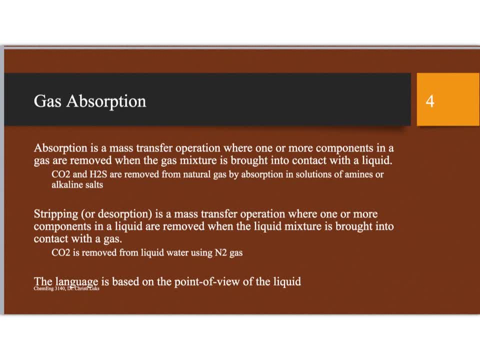 Similarly, stripping could be done when we strip CO2 from liquid water by bringing in another gas, such as nitrogen gas. In either case, the language used is from the point of view of the liquid. okay, If the liquid molecules are more close together, they're going to be our point of view. 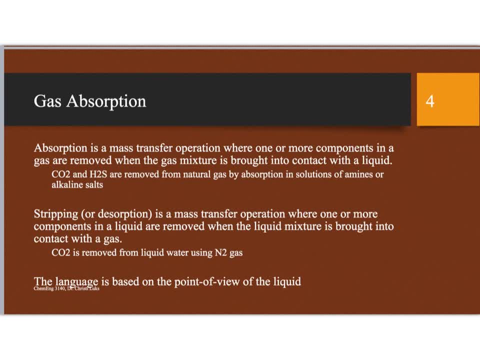 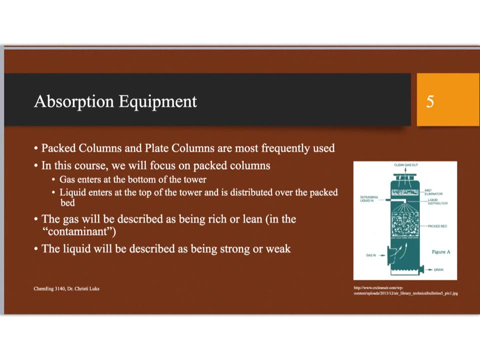 So in the case of being absorbed, the liquid is absorbing the contaminant out of the gas, and stripping the liquid is having material stripped from it. There's a lot of different kinds of equipment that can be used. Most frequently we're going to use packed columns. 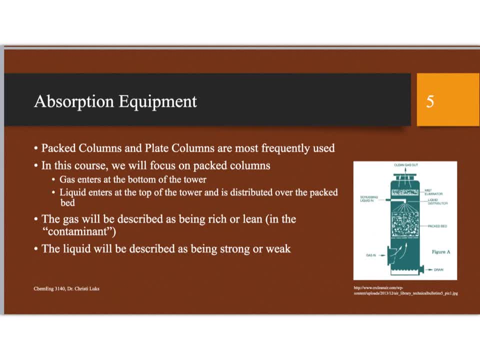 most frequently we're going to use packed columns or plate columns. Our course focuses on the packed columns. Now, in a packed column, basically, the gas will enter the bottom of the tower and liquid will enter the top and they pass through a packing. 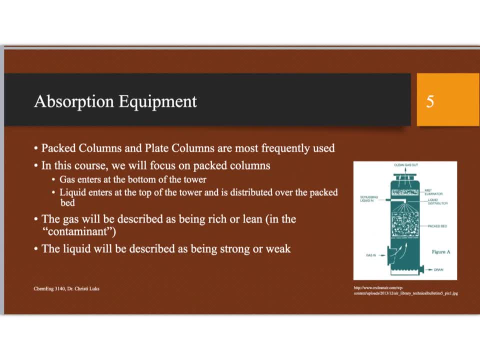 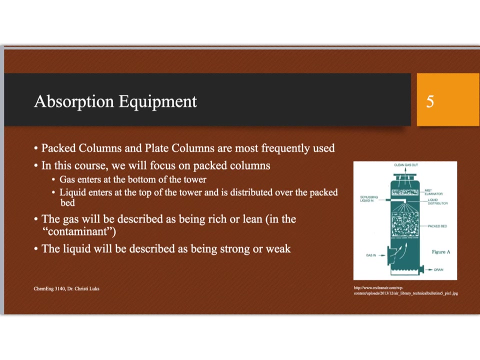 which you can see over to the right. By just geometry and gravitational pull, the gas will tend to rise, the liquid will tend to fall and the packing helps to distribute these so that they mix as fully as possible. We are going to describe the gas as being lean or rich in the contaminant. 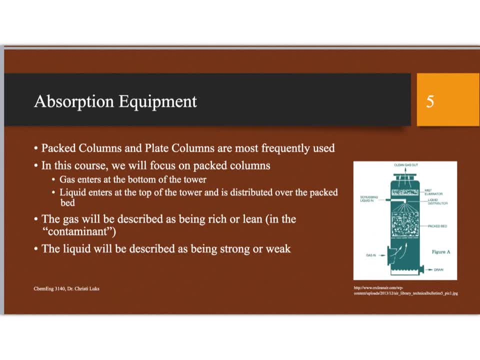 So if it's a rich mixture, it has a lot of the contaminant. A lean mixture has very little of the contaminant. When we talk about the liquid, we're going to talk about it as being strong or weak. Okay, some minor differences in language. 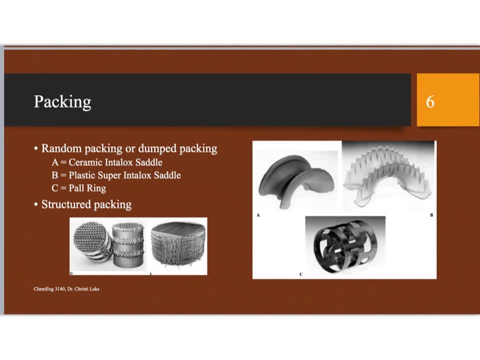 I've shown here a couple of pictures of types of packing. They can be random packing. These pictures that are on your right are showing you samples of random or dumped packing, And you would have thousands of these that would just be dumped together in the column. 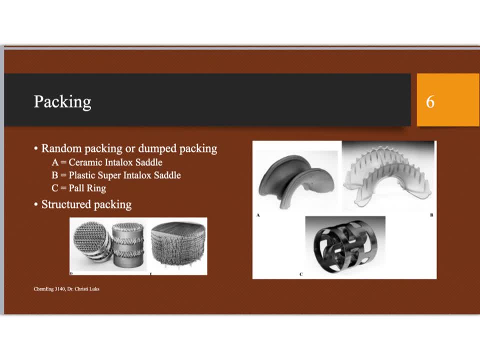 on some sort of grid surface that would allow the gas and the liquid to pass through And these, ideally, will just randomly distribute themselves, so that we don't get any bad flow patterns. Now, we'll be talking about those in the next video lesson.